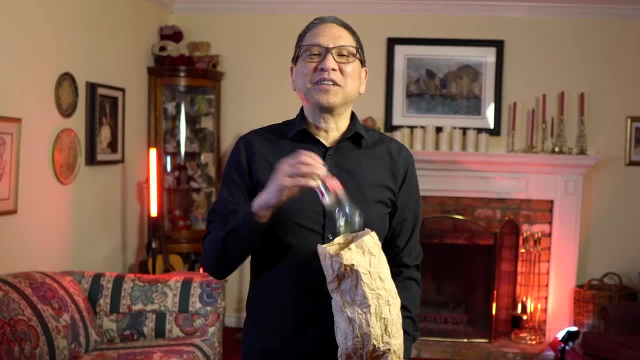 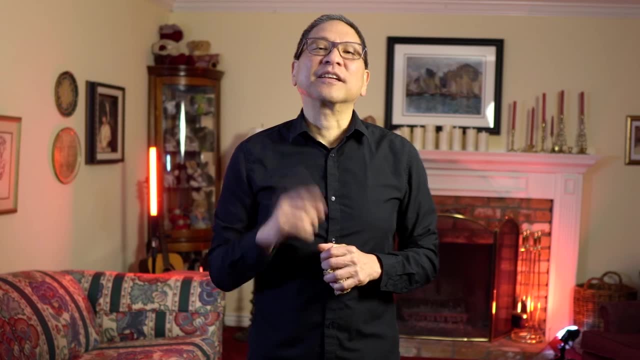 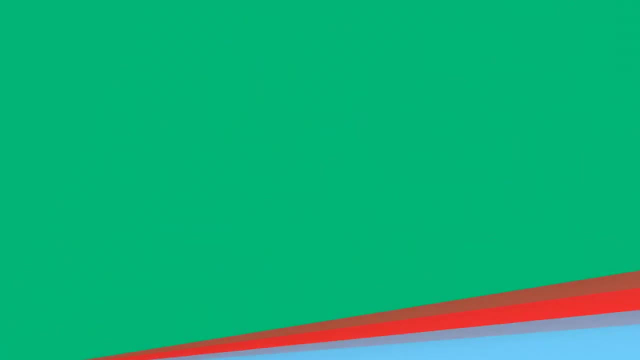 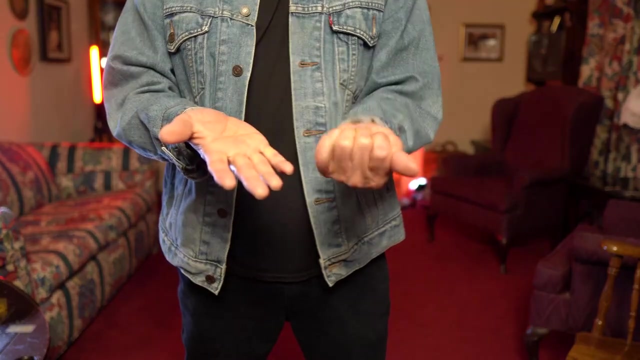 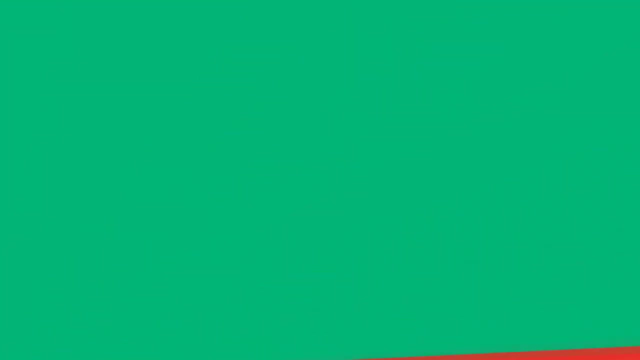 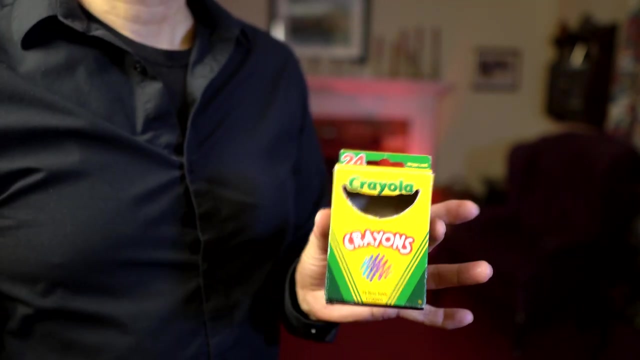 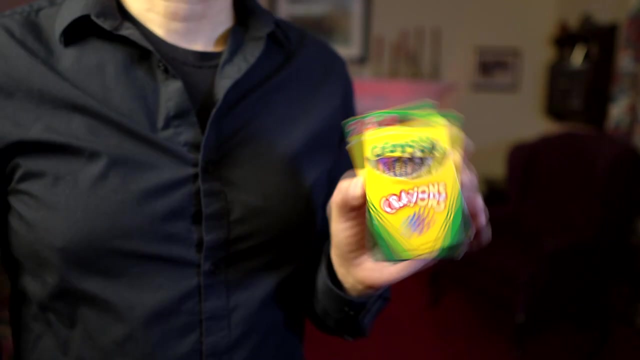 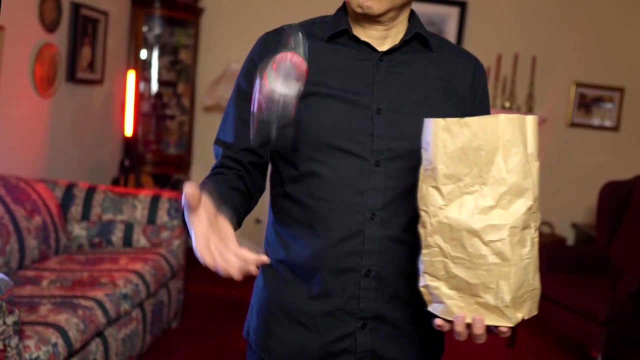 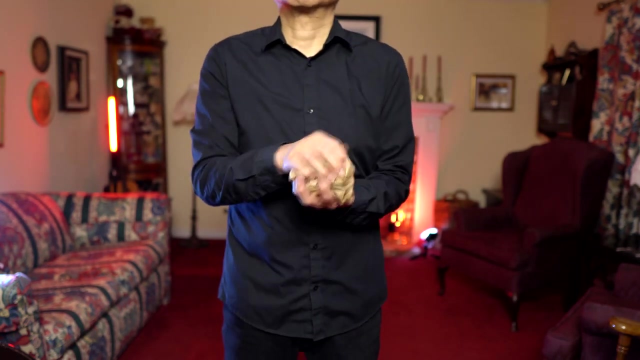 I'm going to teach you how to make things disappear just like magic. First I'm going to show you the tricks, then I'll show you how to do them. Let's get started. I'm going to show you how to make things disappear. 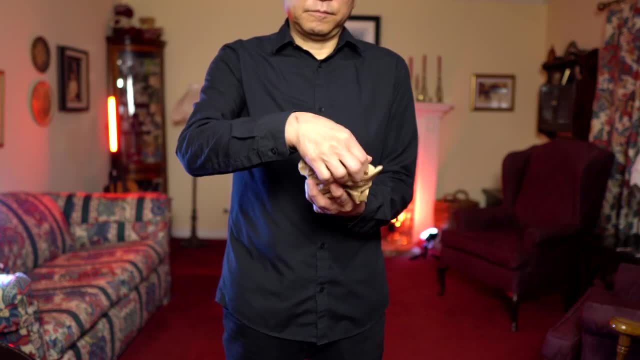 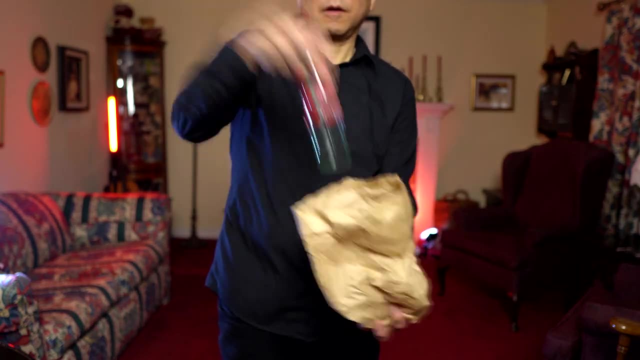 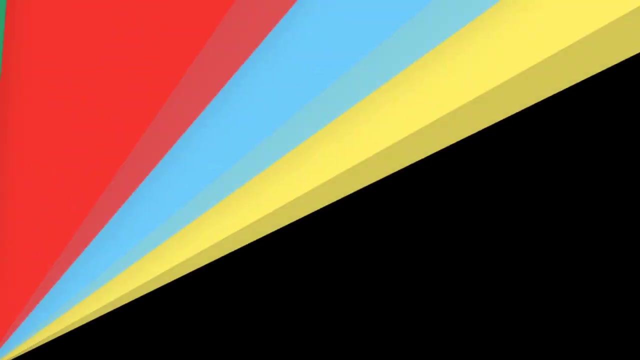 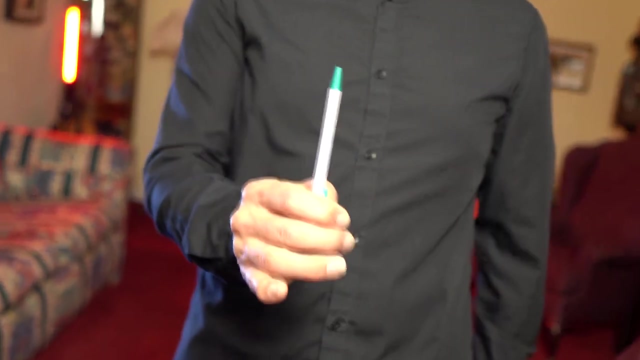 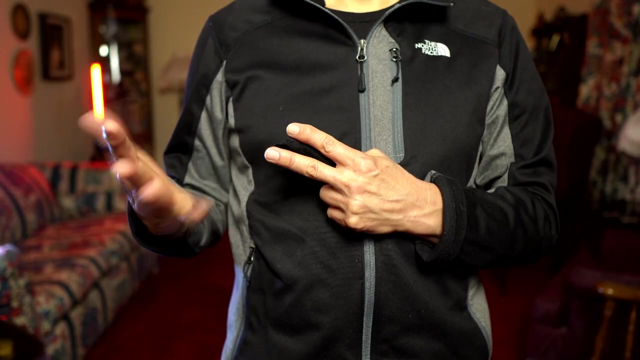 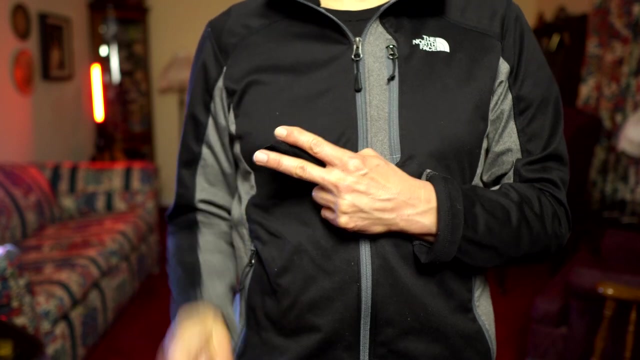 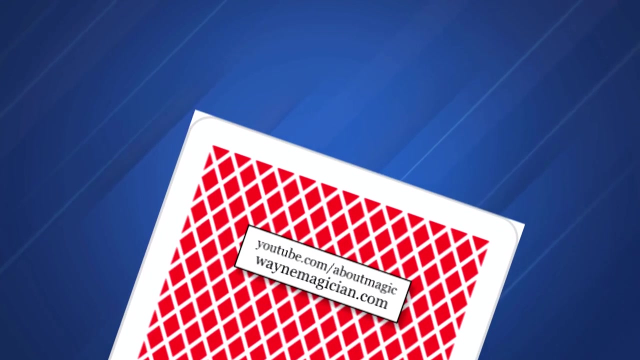 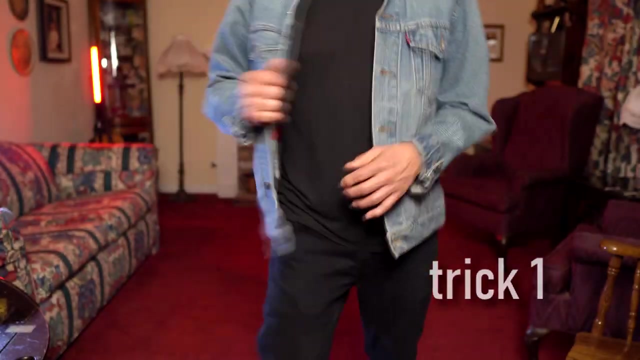 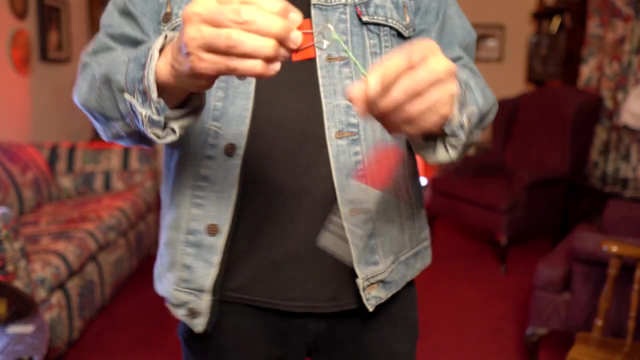 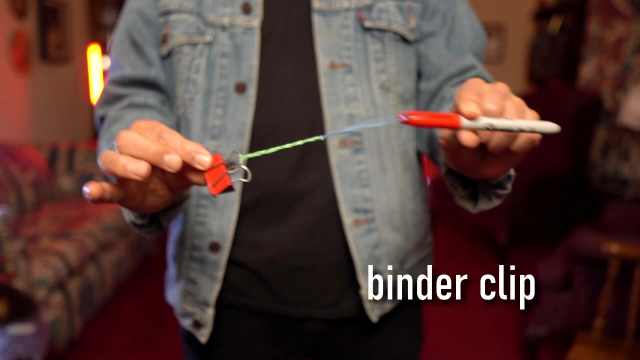 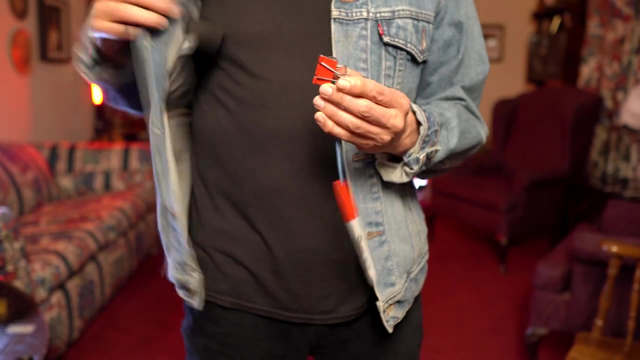 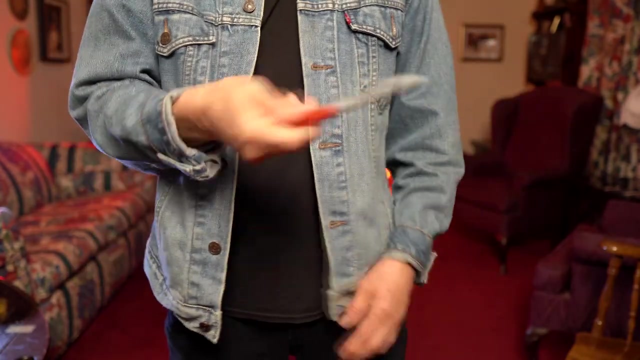 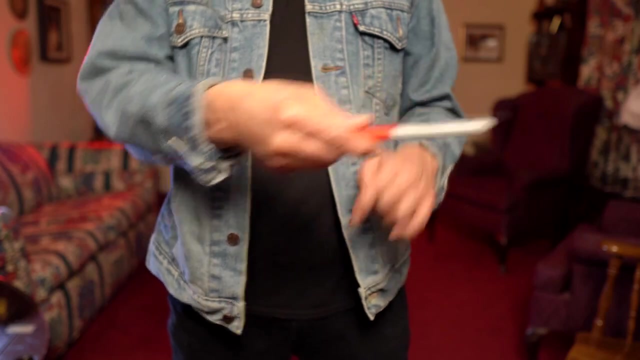 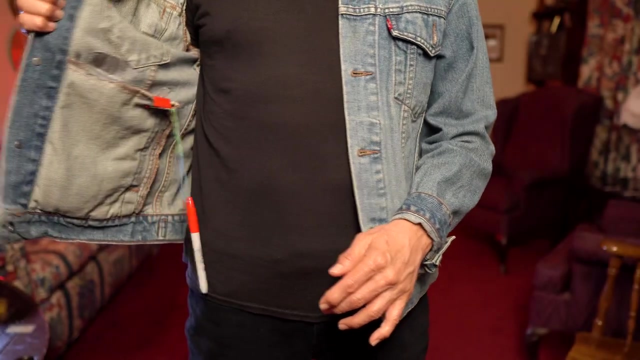 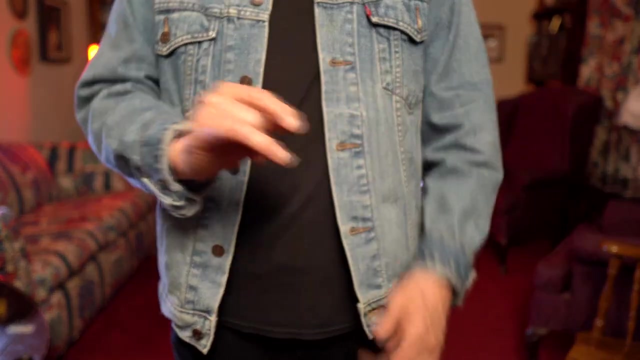 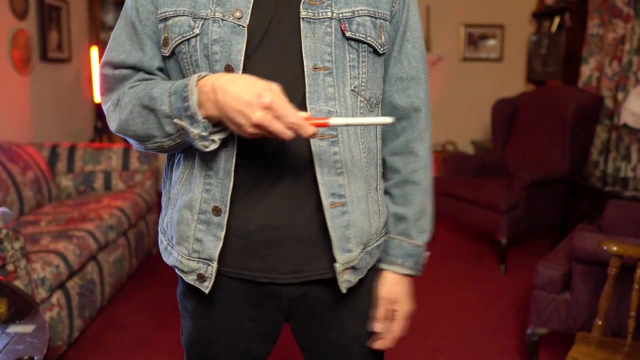 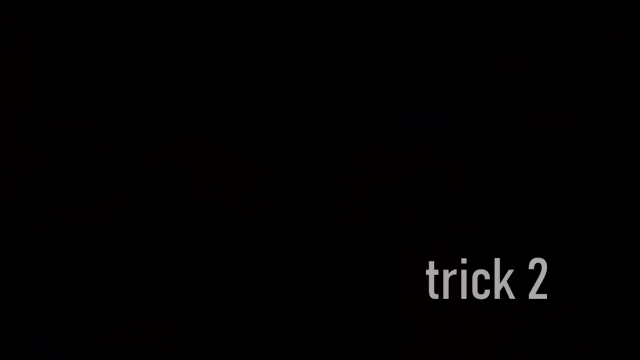 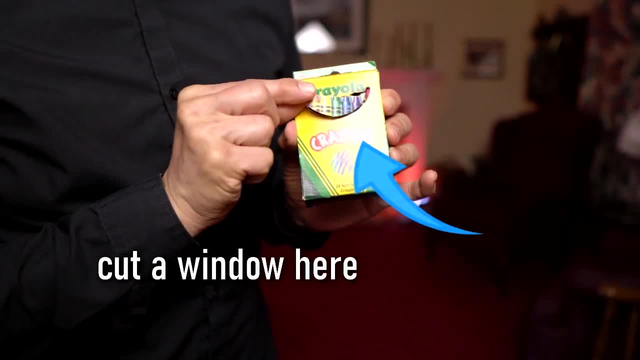 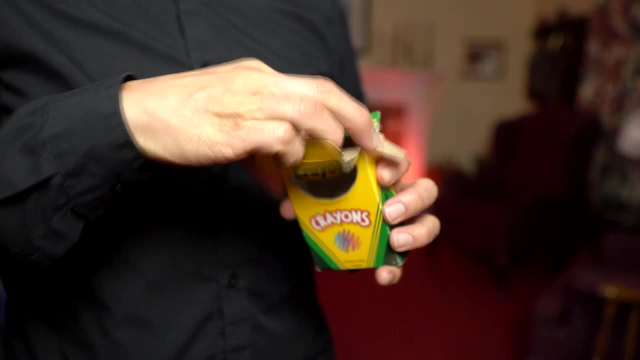 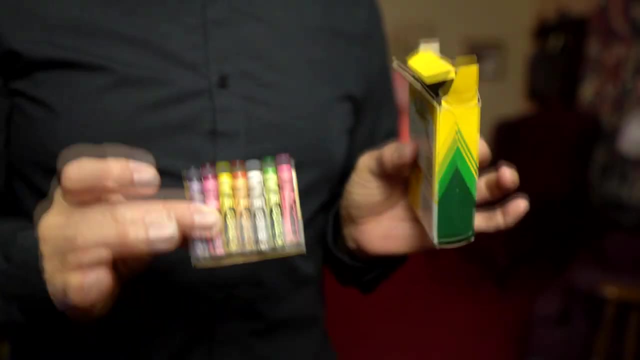 I'm going to show you how to make places disappear. Here's what it's going to look like: Half crayons taped together. If your box is a single thickness of crayons, you don't need to do what I do here, but I 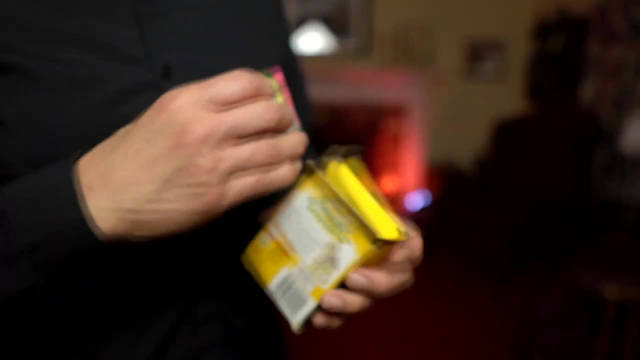 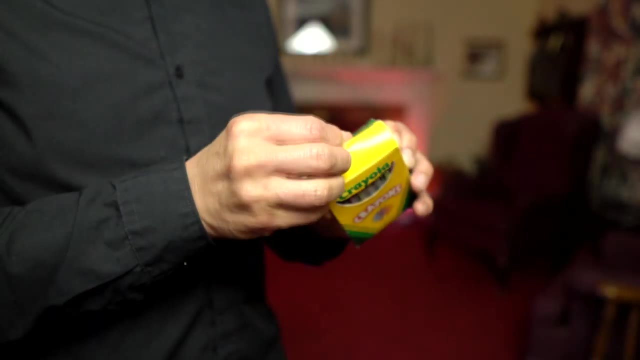 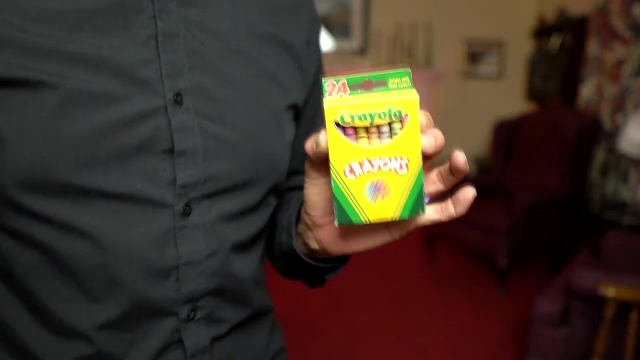 made a spacer out of cardboard here and this is your gimmick- goes into the box. you hold the sides here, close the box. the crayons disappear. you put your hand in front briefly and as you do this, you're letting the crayons drop right there. 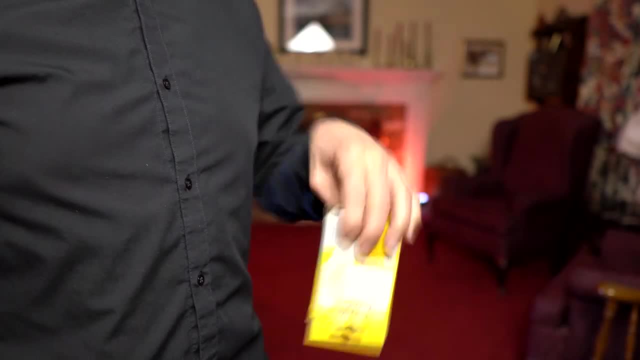 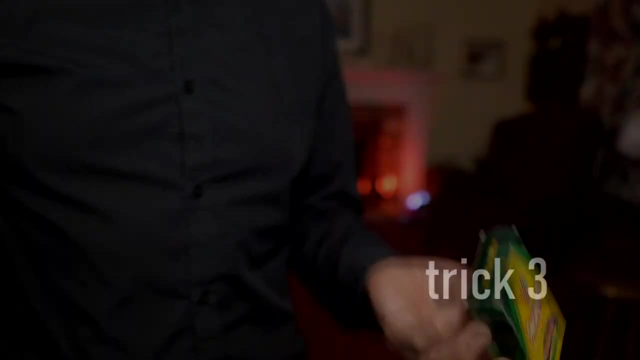 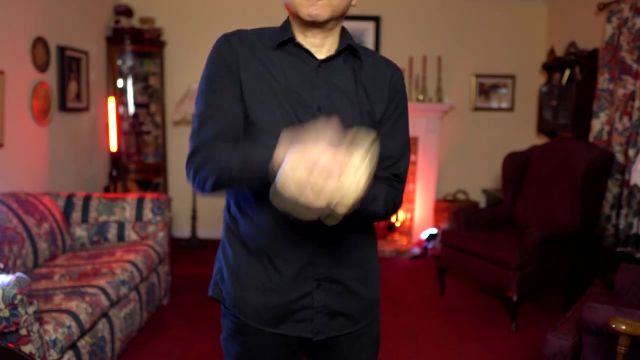 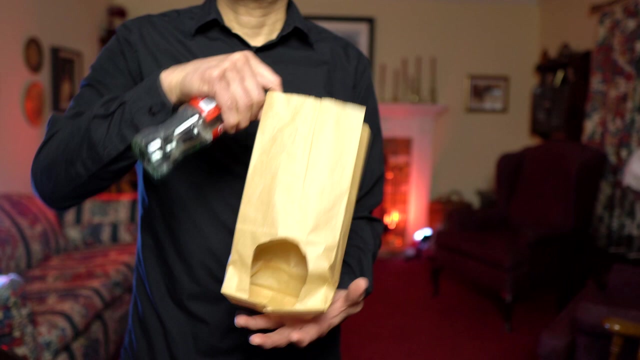 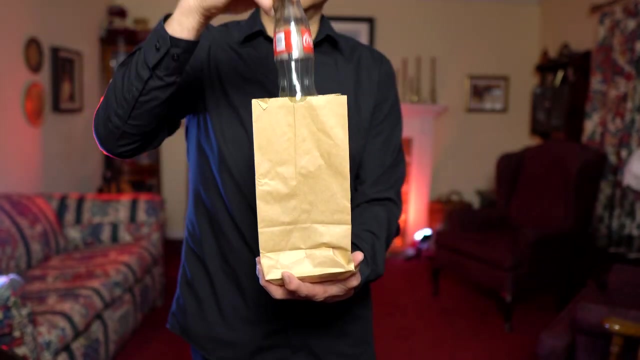 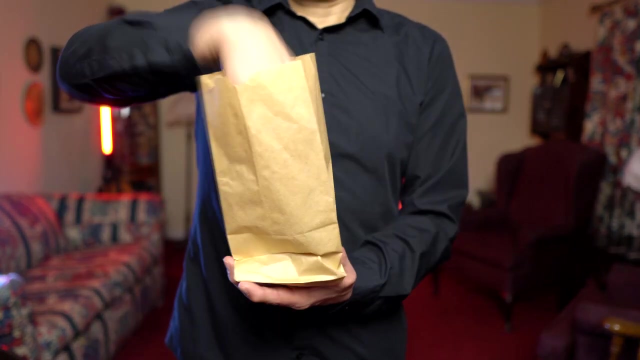 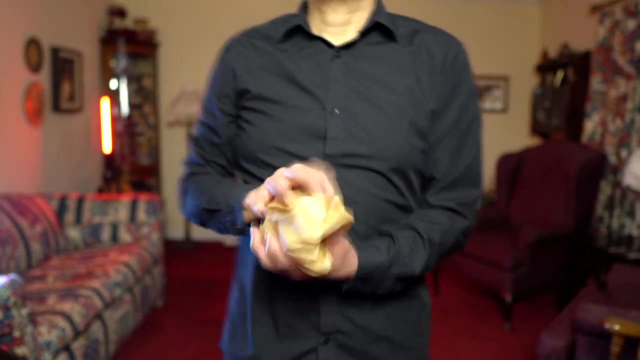 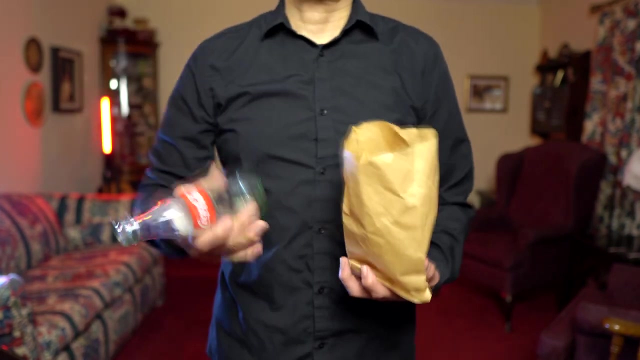 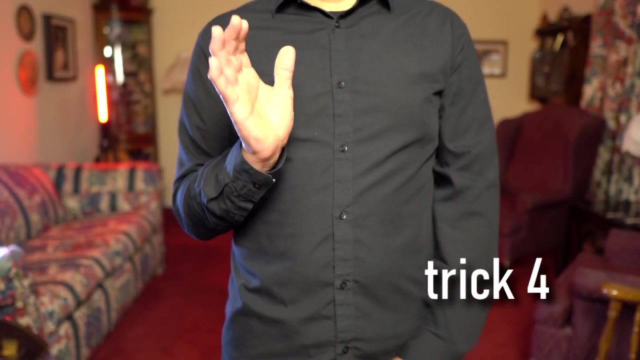 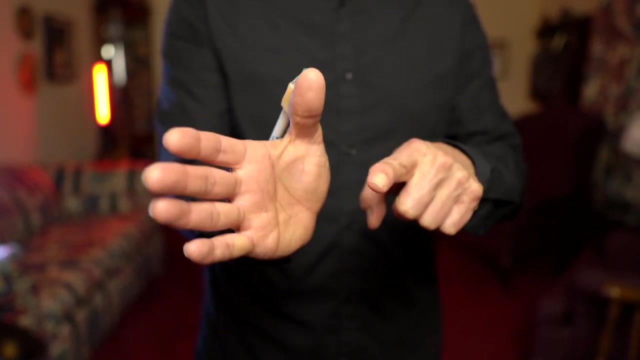 bring it back, turn it over, gravity brings it back. and then just grab it on the sides and the crayons are back. and then just grab it on the sides and the crayons are back. so so The pen is attached to the thumb, so you flip it like this: 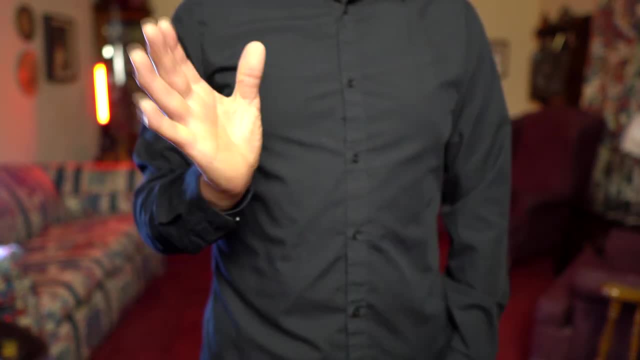 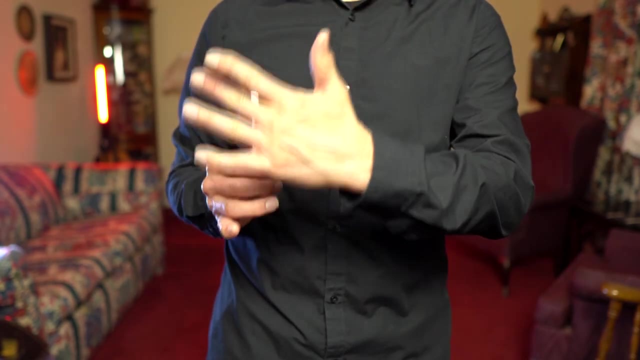 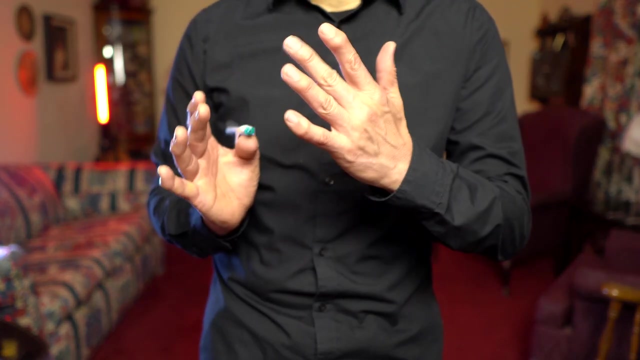 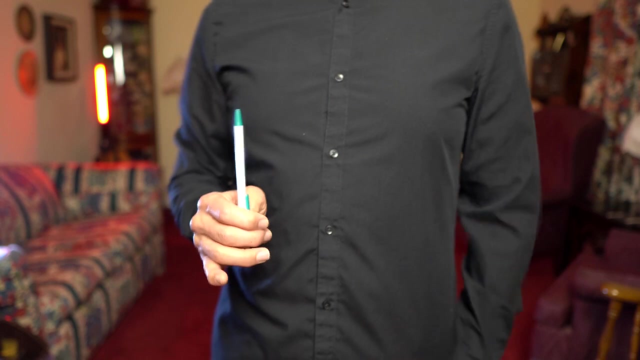 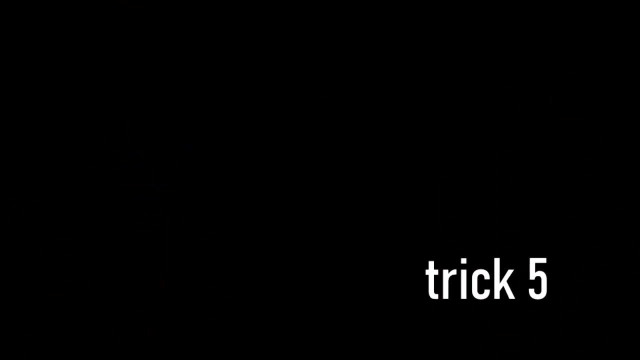 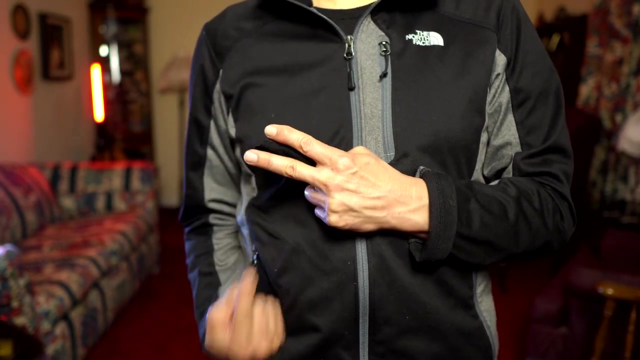 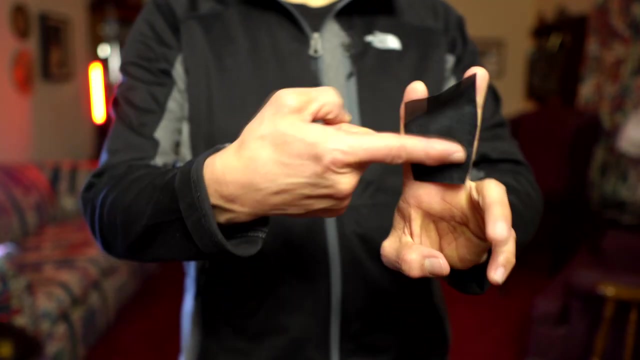 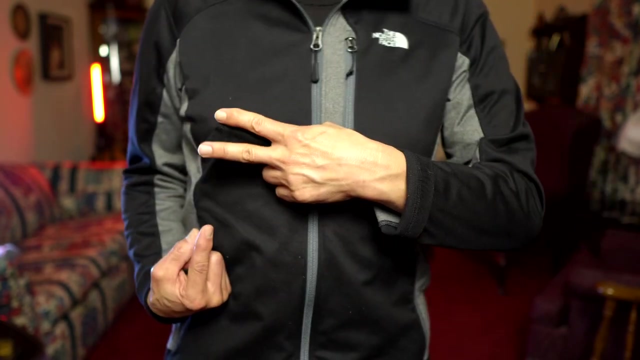 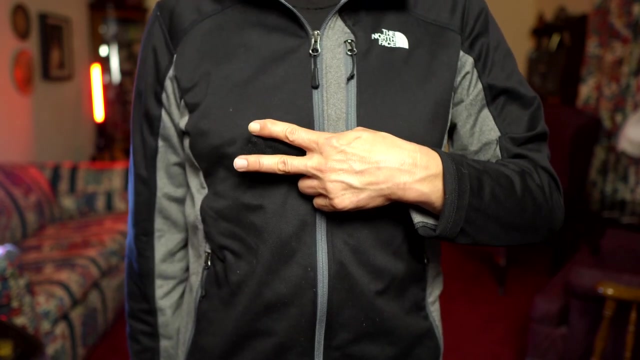 I used a Band-Aid so the tape could extend to the front. The pen is along the back here, so when you use the hand as a cover, the pen vanishes. and to bring it back It's done. Thank you for watching.